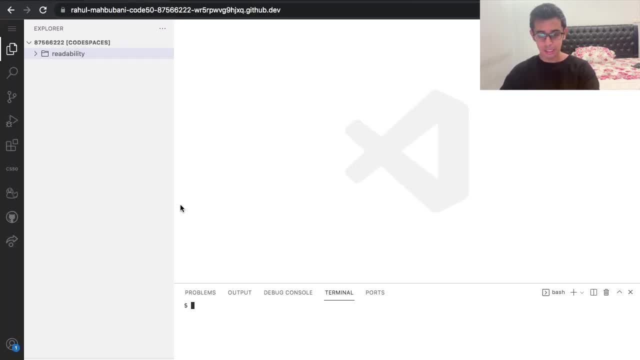 the instructions step by step. So first it says to type cd- and this is just my vs code here: empty cd. okay. and then it tells us to copy this. okay, I'm just going to do exactly what they say. and then it says to unzip: okay, it's going to copy and paste what they tell me to do and rm, and then. 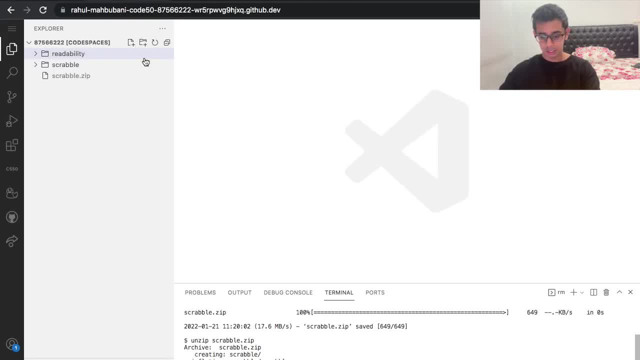 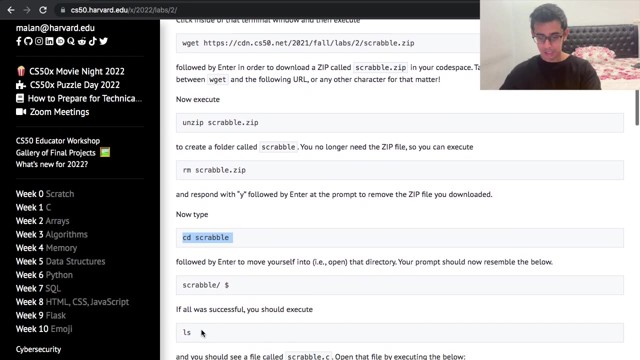 type y- okay. and then type y, enter okay. finally they say: to do cd Scrabble- okay. again I'm just copying and pasting step by step what they tell me to do. and finally they say okay, type ls, ls, okay. and then they say: to do cd Scrabble- okay. and then they say: to do cd Scrabble- okay. and then 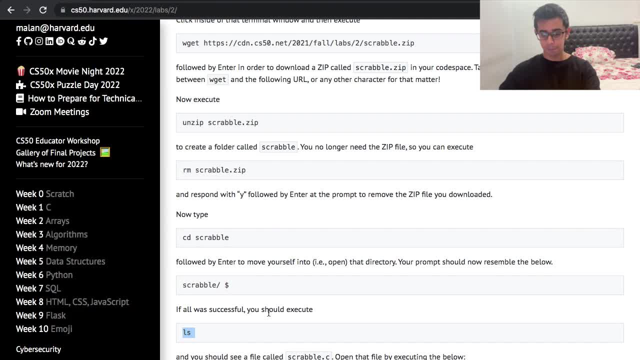 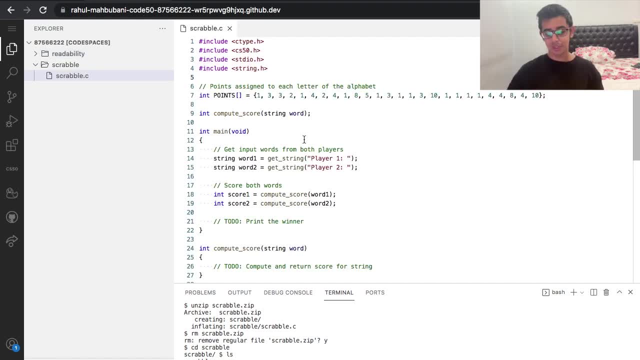 and scrabblec shows up. so that's a good sign. and then we do code scrabblec- okay, and now lots of distribution code comes up. um, so this is the code that they give us when we just follow the instructions on their page. so there's distribution code, or code that csft gives to us- okay, um, but 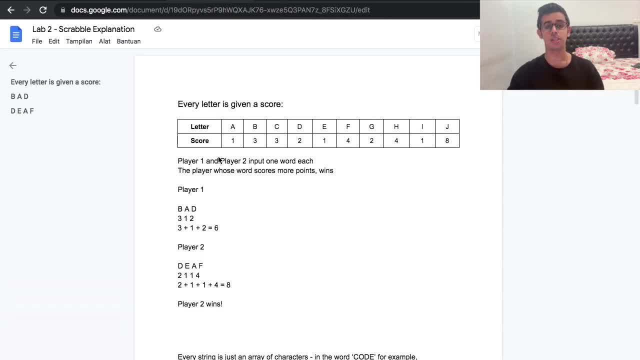 before we jump into that, let's first- uh, let's first understand what scrabble is actually about, what the program is. so here's how it works. every letter is given a score. so letter a is worth one point, b is worth three points, c is worth three points, and so on and so forth. so how it works is: 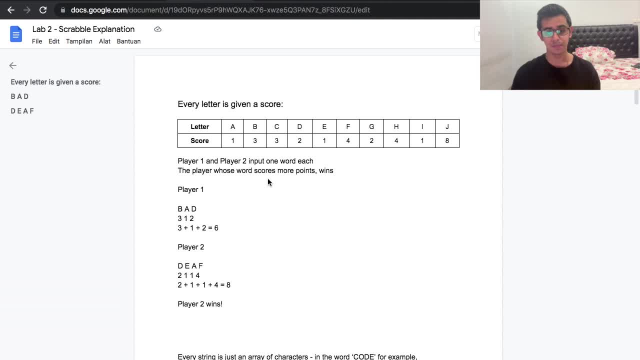 both players, player one and player two, will input a word and the player whose word scores more points wins the game. okay, so let me just give a quick example here. so let's say player one puts in the word bad, so here bad b is worth three points a. 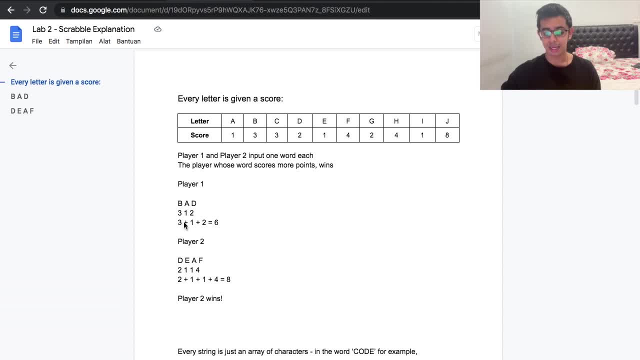 is worth one point and d is worth two points. that gives player one a total of six points. player two puts in the word def, so d is worth two points, e is worth one point, a is worth one point and f is worth four points. so the total score is eight points. so here we can see player two. 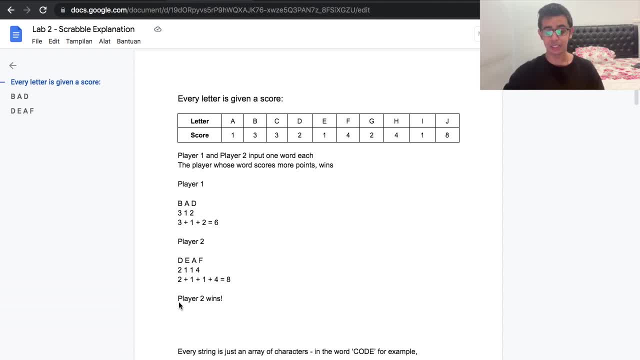 has more points than player one, so the computer should print out: player two wins, okay. so this is a very basic explanation and that's what we have so far. that's what we have to do now. let's take a look at the distribution code that they give us. so first things first. we see 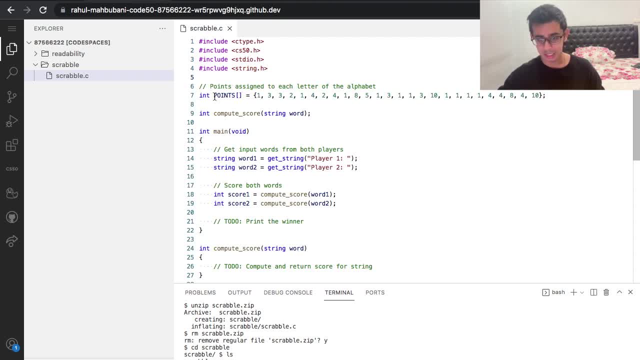 here an array called points, which has ins: okay, and here we can see that this is the points assigned to each letter of the alphabet. okay, so here in the zeroth index, points zero is one, which means that a is worth one point, and in points one, the first index is three, which means b is worth three points. 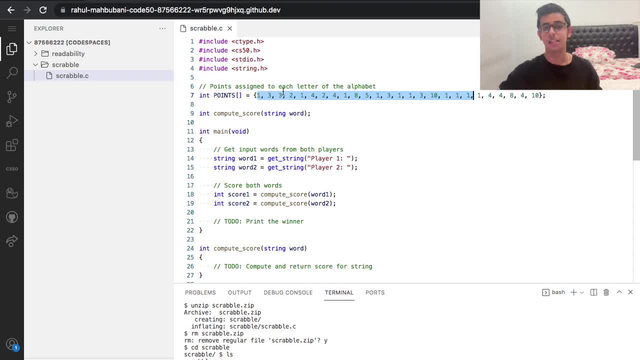 to each letter. so a is one, b is three, c is three, and so on and so forth. right, as we said earlier in this talk. okay, so this is the array that they give us and next up we have a prototype here, a function called compute score that takes in a string called word and outputs an integer. okay, 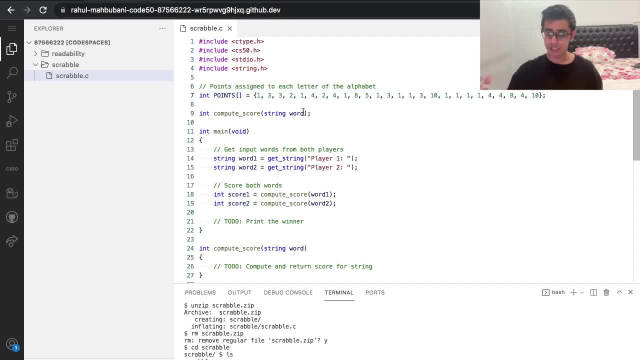 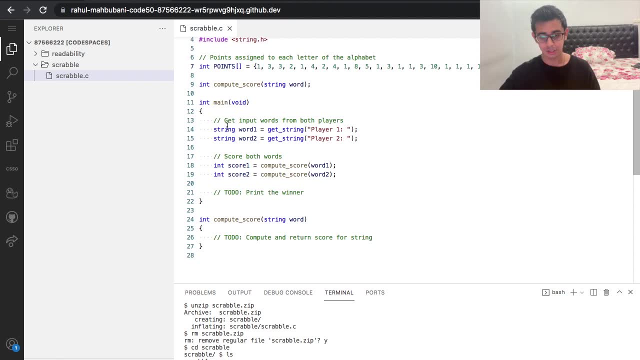 and so far this makes sense, because the player is going to give us a word, so that's the input and it's going to output an int, which is the score. right, okay, so let's go. i'm just going through the code step by step. by the way, we don't have to write. 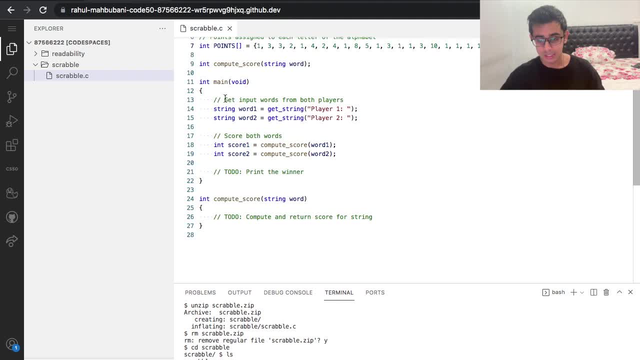 this code. this is the code already given to us. so next thing you do is get input from both players. okay, and how we do that is using the get string function, if you remember from earlier problem sets. so string word one equals to get string, getting some input from the user, and the same thing. 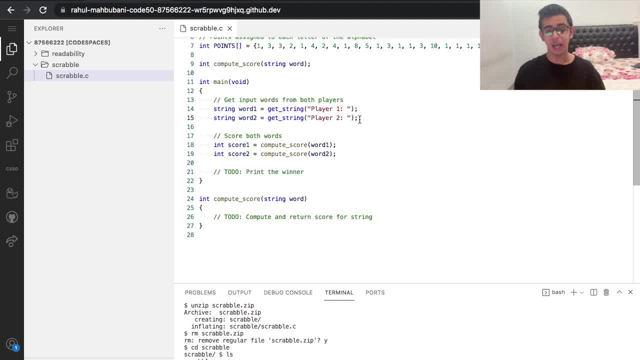 for word two. so we're getting two inputs, one from player one and one from player two, and that's where they type in the word, and next thing we have to do is score both words. right? so int score one equals compute score word one. and this is the prototype we saw earlier, right? so we have to write this function. 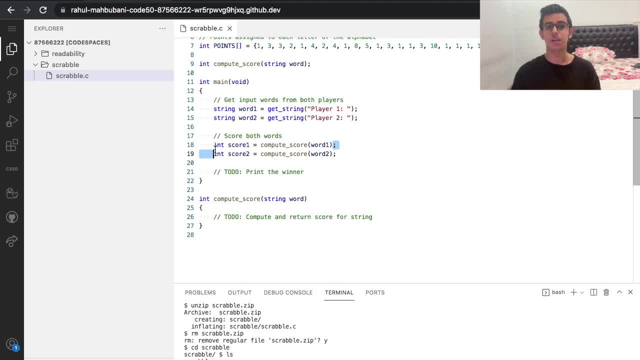 so they don't tell us how to compute the score. we have to write the program that completes the score, right, and finally we have to print the winner, okay, so first thing we have to do here is let's actually write the function. so how do we go about that when the player and the 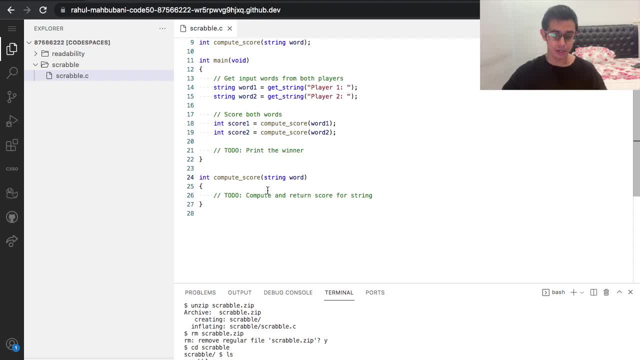 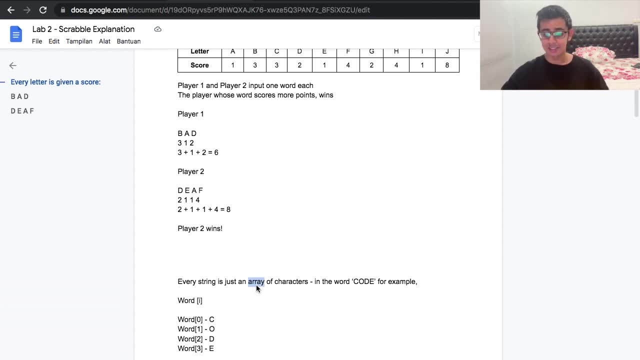 user input a word, we need a specific score to be given to that word, right? so let's take a look here. we should remember that every string is just an array of characters, right? if you remember from the lecture, every string is just an array of characters. so let's take an example here: the 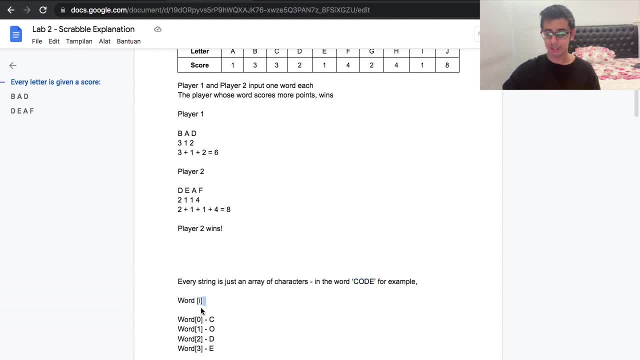 word code. so code is a string. right, the word code is a string, but it's actually just an array of characters. so let's just say: um, this is an array called word, and in the zeroth index will be the letter c and the first index will be the letter o and the second 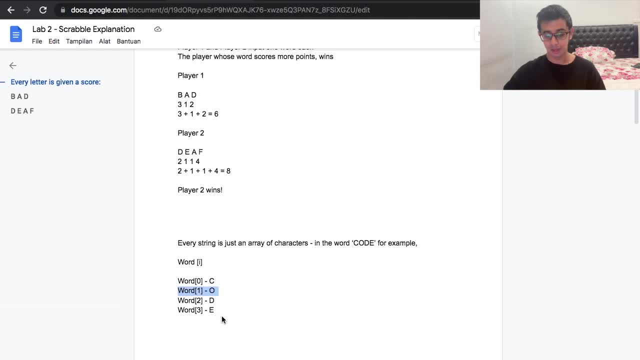 index will be the letter d and the third index will be the letter e, which makes up the word code. right? so every character has its own index here. so every character is an index in the array and every string is just an array of characters, as we can see here. 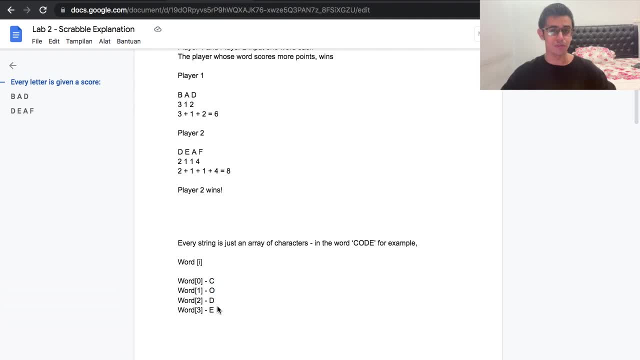 okay. so how do we go about calculating the score, then, of each word? well, it will make sense that we loop through every character in the word, every, every index in the array to find out the score of each letter. right, so we go through them one by one, again and again, until the end of the word. 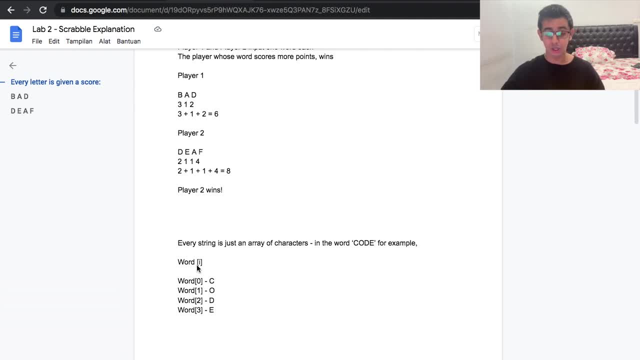 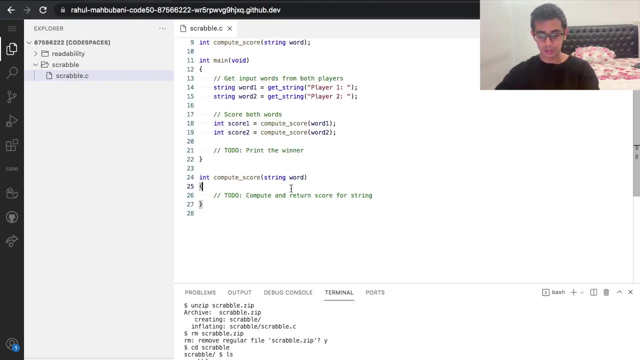 so it sounds like we need to use some sort of loop to do this, to go over each character one by one, and let's go ahead and do that. so let's code here and here. we know we can use a for loop. so for, let's just set an index, let's call it zero i, let's initialize it to zero. i equals to zero. 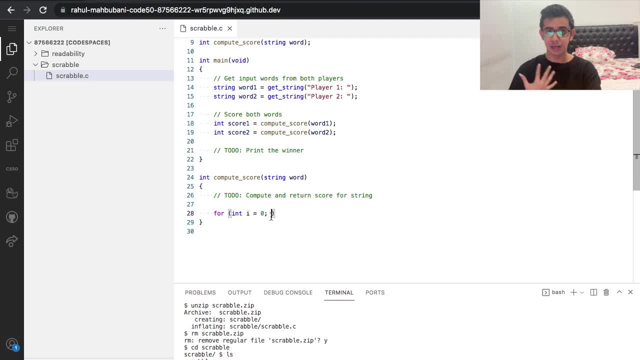 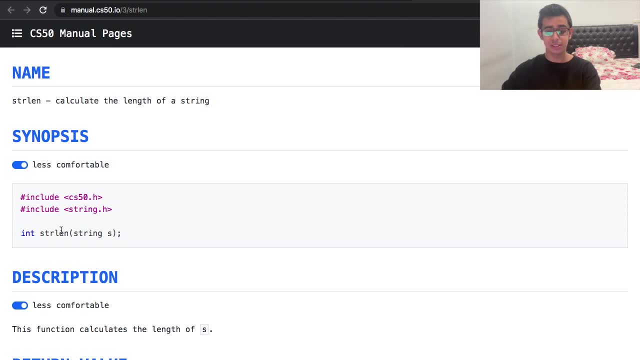 and i equals to zero and we need to keep on going along the length of the word and, if you remember, there is actually a function that's that lets us do this sterling right. so let's use this function, which is under string dot h, which tells us the length of the string. okay, 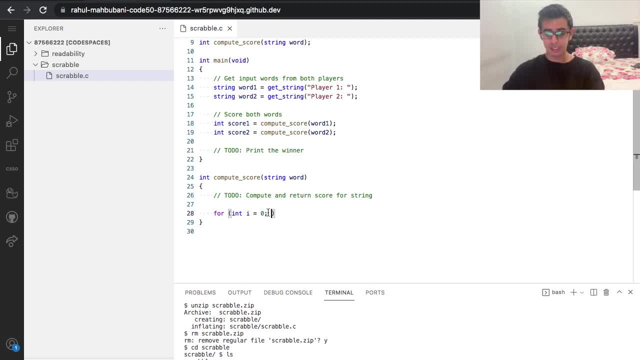 so if you remember how a for loop is is arranged, it's first you initialize it to something right and then we give it a condition: keep on going as long as. so we want to keep on going as long as i is less than the length of the string called word. right, so i is less than sterling of words. 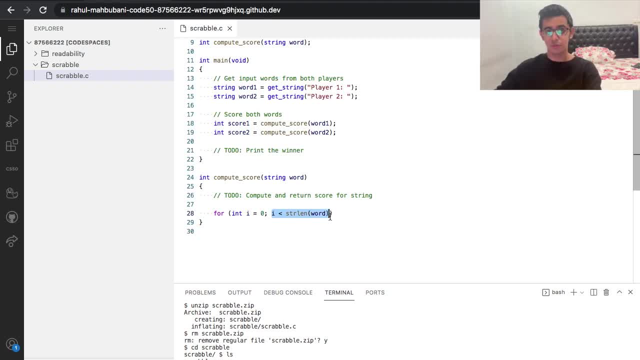 so keep on going. keep on going as long as i is less than the string length of a word, and we want to keep on going one, so we do i plus plus. so what it says here is: if i equals to zero, we initialize it to zero. keep on going as long as there's still letters in that word, and we want to go one by one, so i plus. 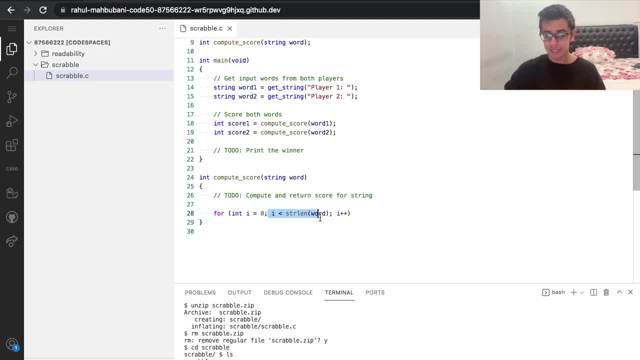 plus. so it's initialize condition and then the increment. okay, so for this, what we want to do, we want to compute the score right. so first things first. we know we need to have a variable called score to keep track of the score. so let's have an integer. of course, score can either be 0, 1, 2, 3, so 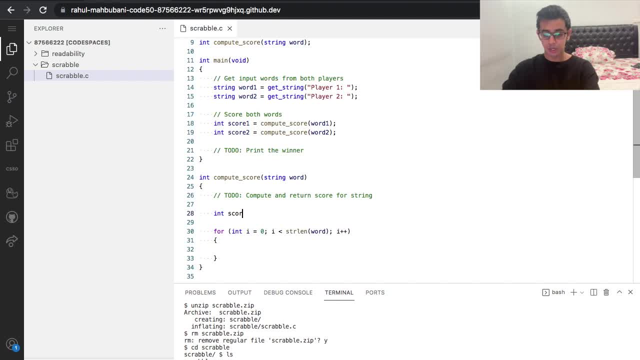 on and so forth. it's not going to be a decimal right. so let's do int score and let's initialize it to zero. let's start to zero, right. so here, when someone types a letter in the computer, what happens? so actually, if you remember from the lecture, every letter has its own position on. 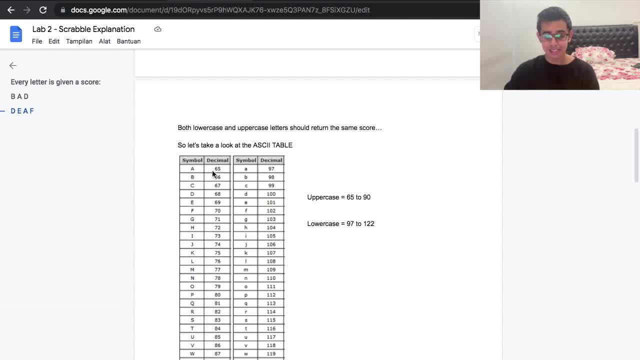 the ascii table right. so we can see here that capital a is 65, capital b is 66, c is 67 and so on and so forth. and this is according to ascii table which the computer uses. but uh, now we can see that actually capital a, uppercase a, is in the 65th position according to ascii, but lowercase a is in the 97th. 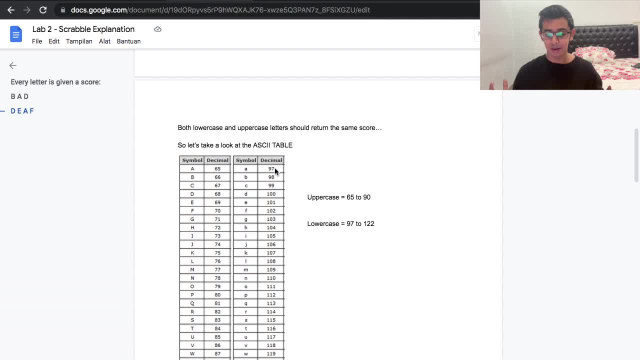 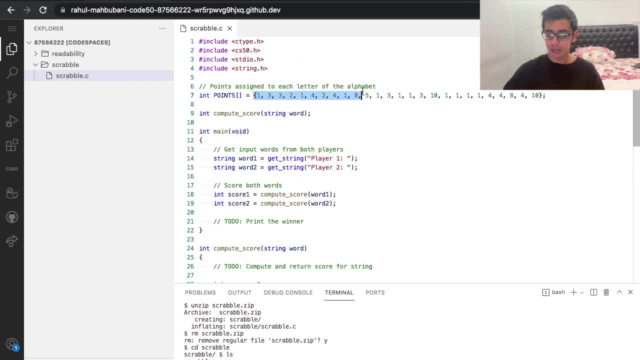 position. so uppercase and lowercase a have different positions in the ascii table. but when we compare it to the array here, the points array, it doesn't matter whether it's capital or lowercase points. a still needs to be in the zeroth index of points right and b whether 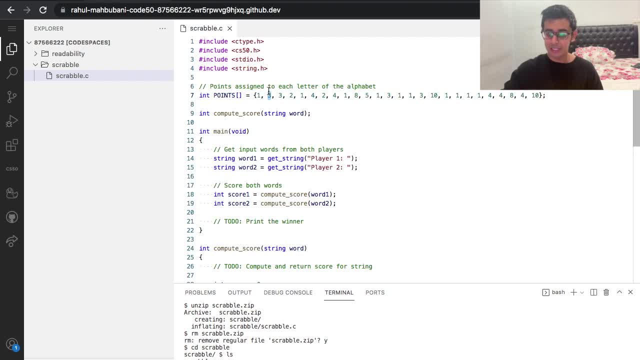 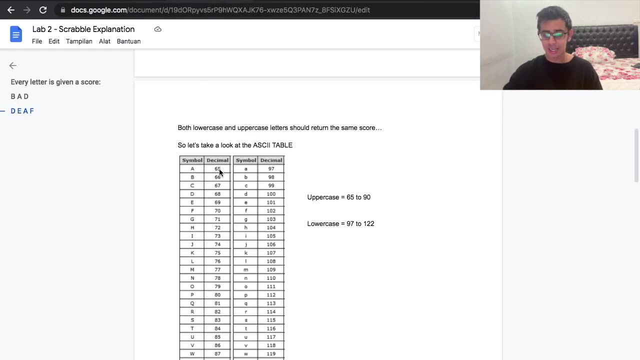 it's uppercase or lowercase doesn't matter. in scrabble we still need it to be in the first index of points, right? so a needs to be in the zeroth index and b needs to be in the first index, and so on and so forth. but according to ascii, uh, it's different: right a is 65 and uppercase a is 65 and lowercase a is 97. 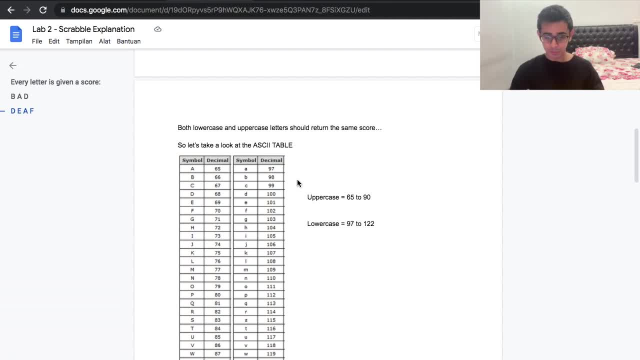 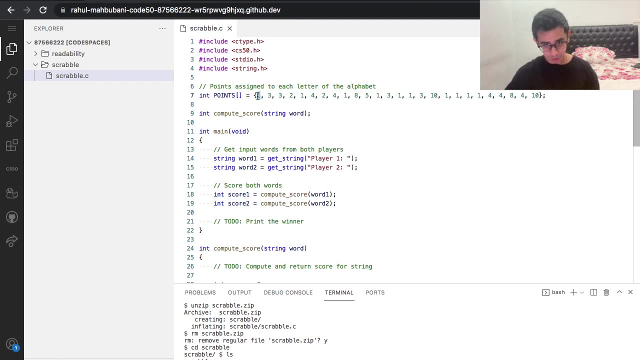 so already, immediately, just like that, we know that we need to treat uppercase and lowercase letters differently, right? so how do we go about doing this? we need to convert it from ascii, from its position in ascii, to its position in the points array. okay, i hope everything makes sense. 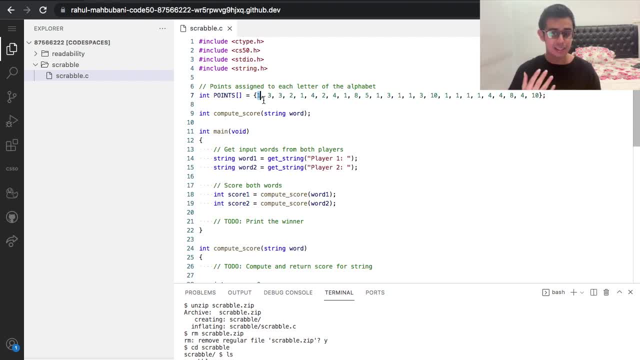 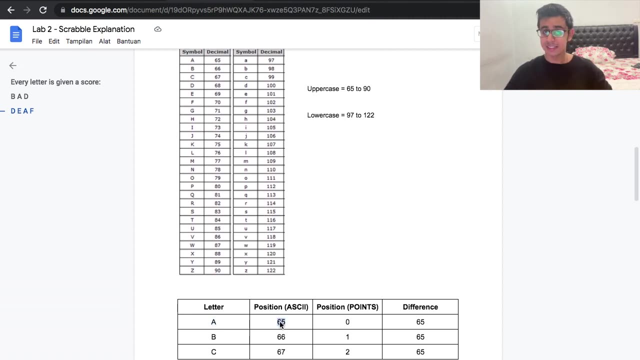 so far and i'll see you in the next video. bye, bye, because the computer, when we type a letter, understands ascii, but here we need to make it equal to the. we need to make it equal to the position in the points array. so how do we go about doing this? well, we know that uppercase a its position, ascii 65. 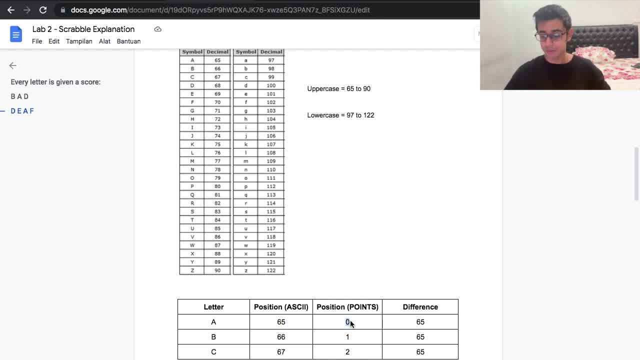 its position in points is zero. right, you can see here: a is in the zeroth index of points, b is 66 in ascii, but in points it's 65 and lowercase a is 67 and lowercase a is 97 and lowercase a is 97. 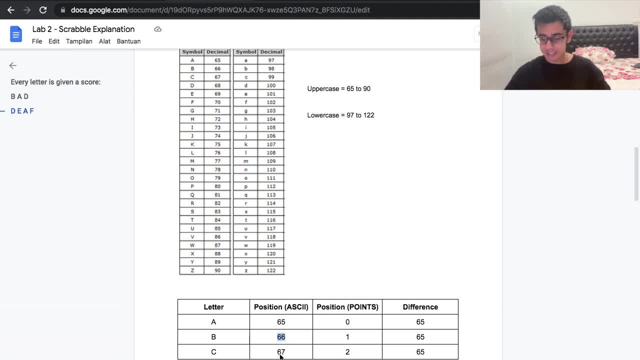 it's in the first index, c, 67th in ascii and second in the points array. so the difference here is always 65, right? so it actually is just ascii minus 65 is where it is in the points array. so in the 65th position of ascii is the same thing as the zeroth index of the array points. 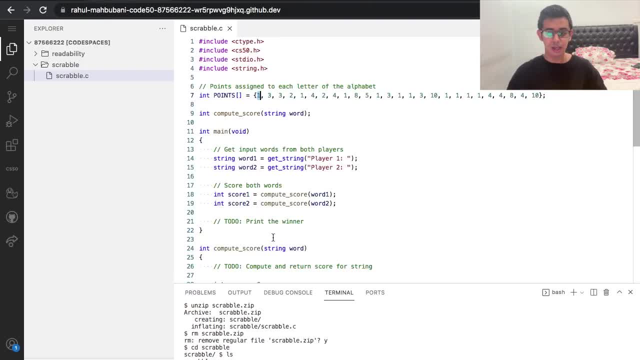 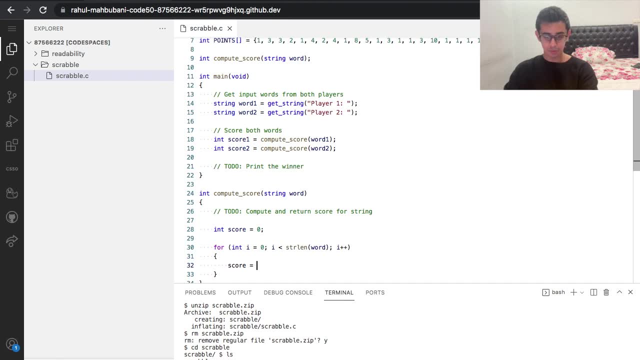 okay, so that makes sense. so let's try to make a formula here for the score. so score equals: what is it? we need to update it every time. so score plus. now, which, uh? which position in the points array should it be? so points, which array should it be here? it should be: whatever the index is in ascii, which is word right minus 65. 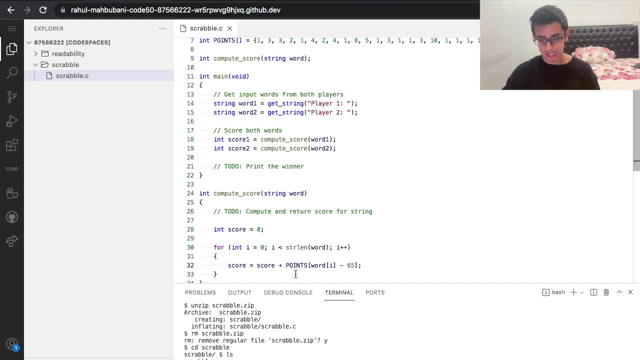 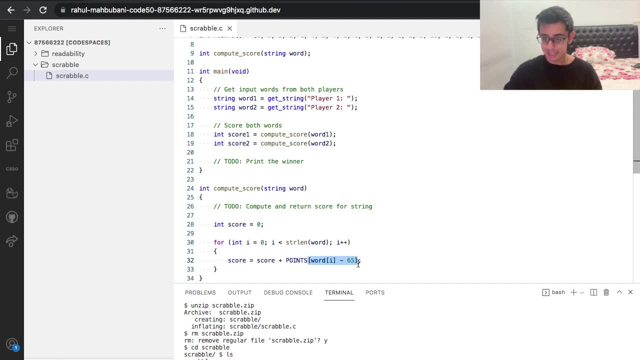 okay, and i hope that makes sense and i'll just explain it once again. so, um, here what the index of points that it takes is. whatever index it actually is from the word minus 65, because this is according to ascii. the index of the word is according to ascii, right? so here? 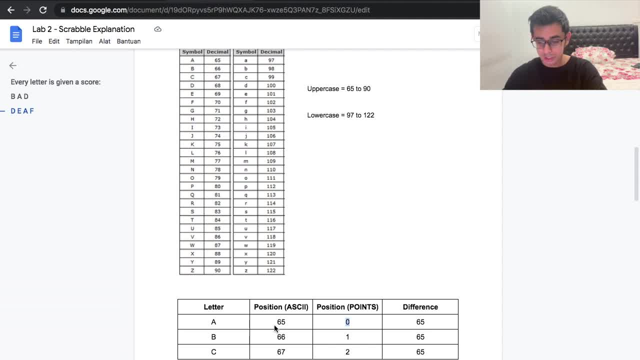 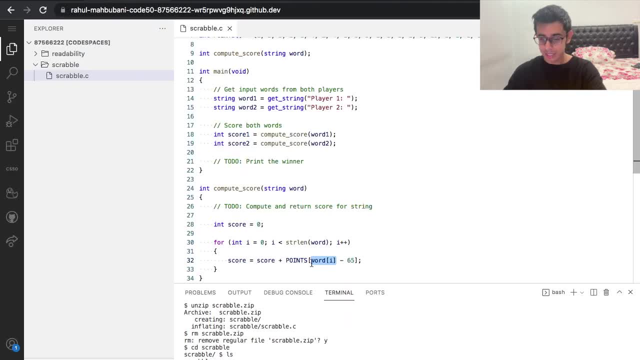 uh, right, like we said, it should be in ascii 65, but in points it's zero. so that's why we need to do whatever it is. whatever, the index of the word is minus 65. so index in ascii minus 65 will give us the index in the points array. okay, i hope that makes sense. 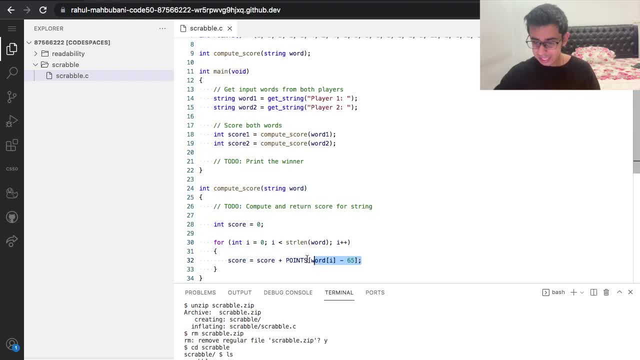 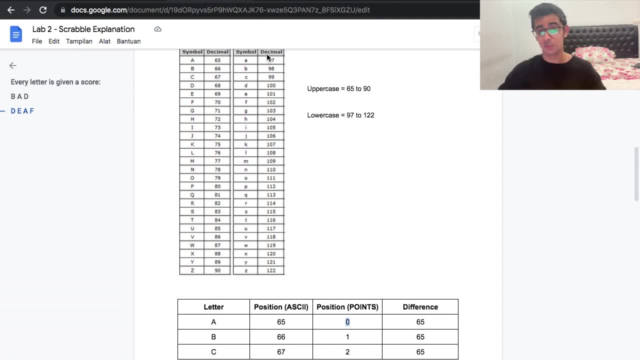 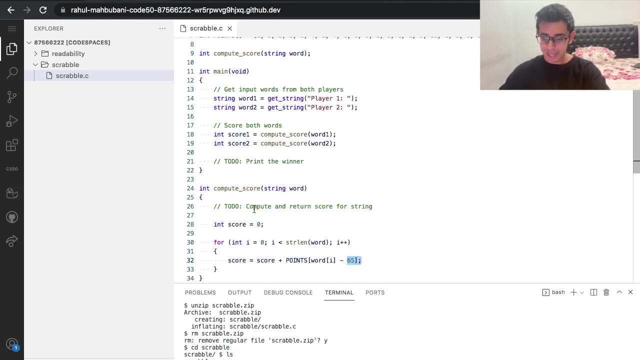 so far. but here we can see that this 65 is actually only applicable for the uppercase letters, because for the lowercase letters we need to treat them differently, right? so how do we tell the computer that this only applies? applies, this only applies if it's an uppercase letter. it sounds like we need to use a condition. 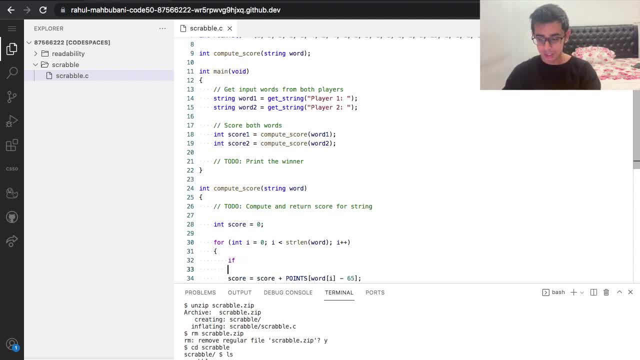 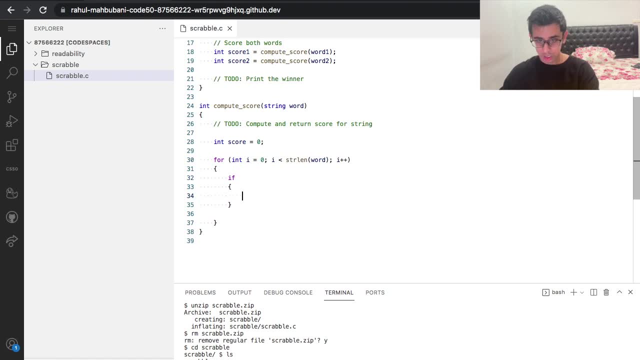 here, which is the if condition, right? so if sorry, let's put that within the if condition here. so if something is true, then this: so if it's an uppercase letter, then we need to subtract 65. so how do we say it's an uppercase letter? well, we see the position here. it's six. 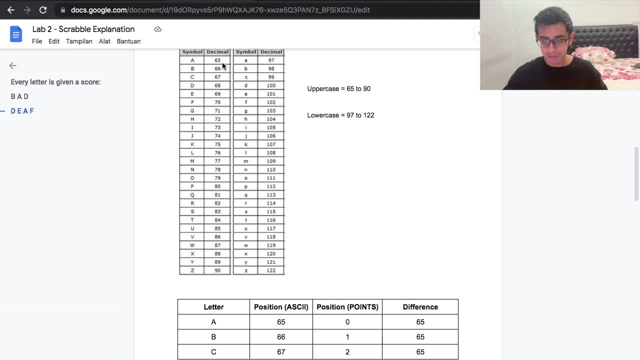 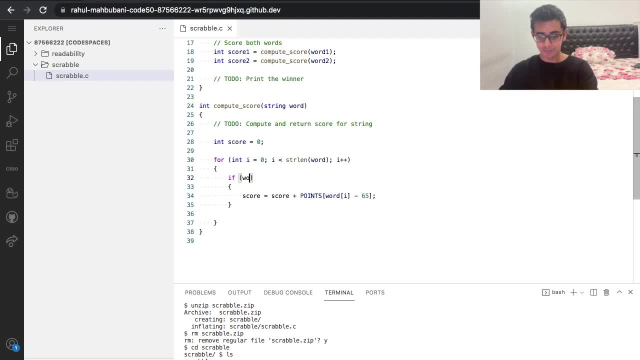 uppercase letters in the ascii are 65 to 90. right uppercase is 65 to 90. okay, so we can simply say: if the index of word is greater than 65, and and how do? how do we say: and in the in the this condition, it's double ampersands. okay, so if 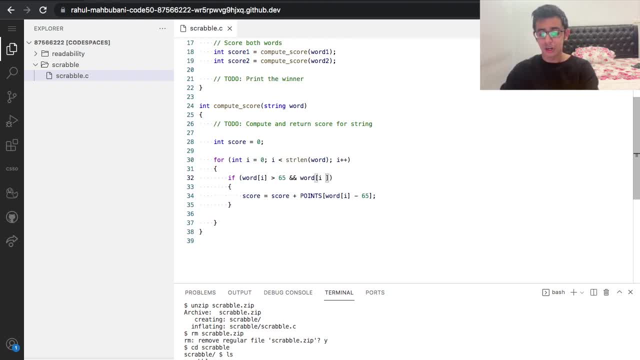 it's less than 65, sorry, if it's less than 65. if it's less than 65, it's greater than 65 and it's less than 90, right? so this is the way you tell the computer that, hey, if it's between 65 and 90, then do this, which makes sense, right? everything makes sense so far. 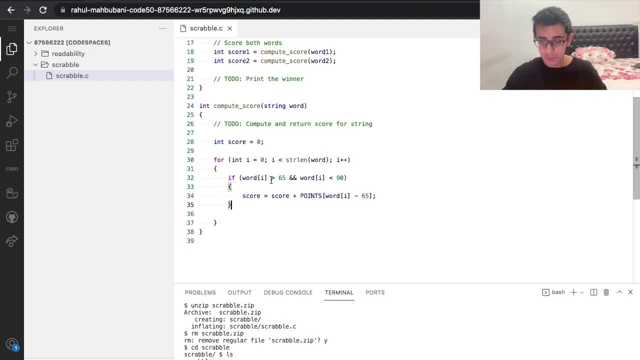 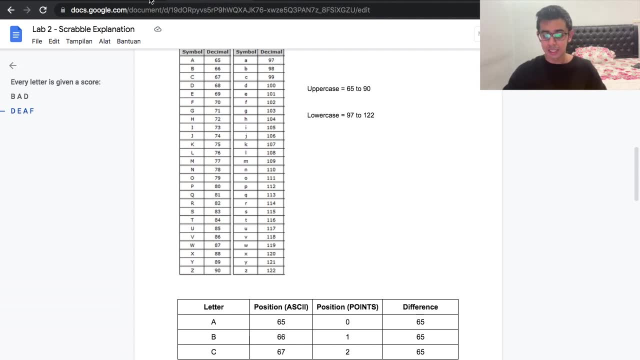 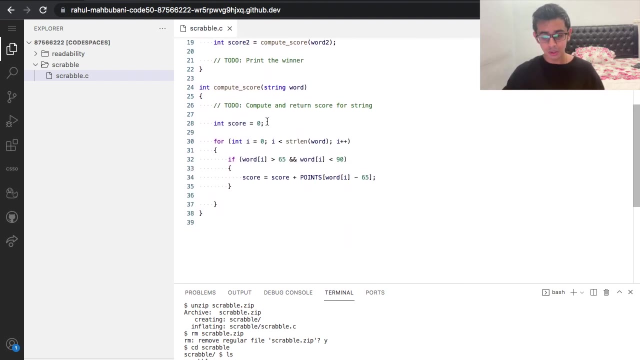 hopefully. but now we need to treat lowercase letters separately again, because here it's 97, a is 97, whereas in our points array a is still 0. whether it's uppercase or lowercase doesn't matter at all. so again now we need to tell the computer: if it's lowercase, then we need to do the same. 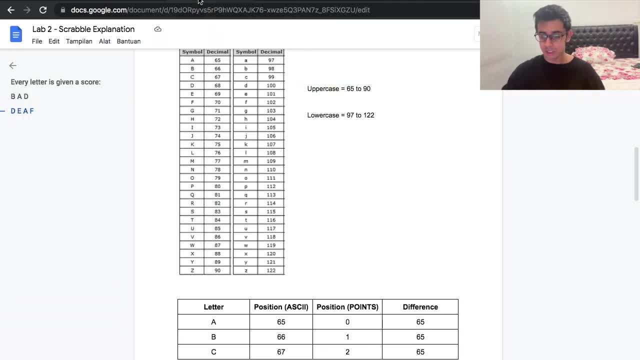 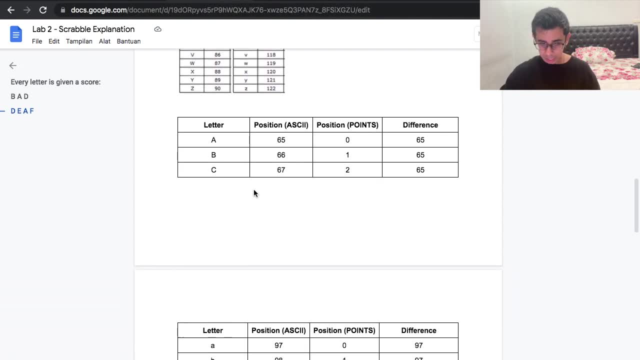 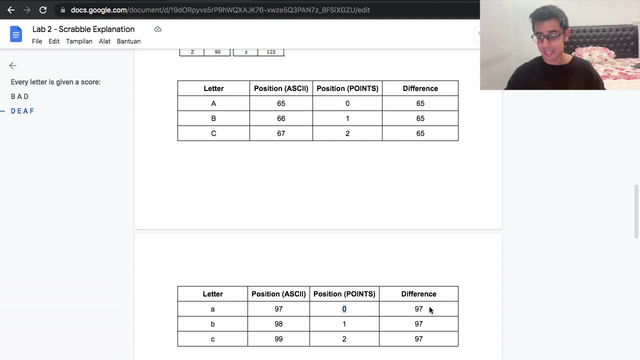 thing. but instead of subtracting 65, how much do you think we should subtract? well, we should subtract. we should subtract 97, right, that makes sense. and here here's how it works. so lowercase a in ascii is 97, but in points it's 0, so the difference is 97.. same goes with b. b is 98. 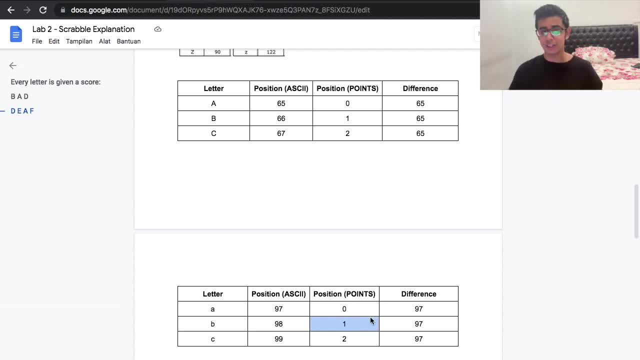 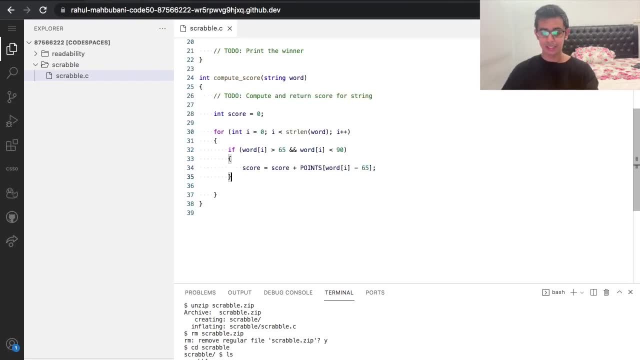 in ascii, but in the points array it's 1.. so the difference here is always going to be 97. so for lowercase letters we need to subtract 97. okay, so hopefully that makes sense. so now we do if, if the index is greater than 97 and it's less than whatever capital z. 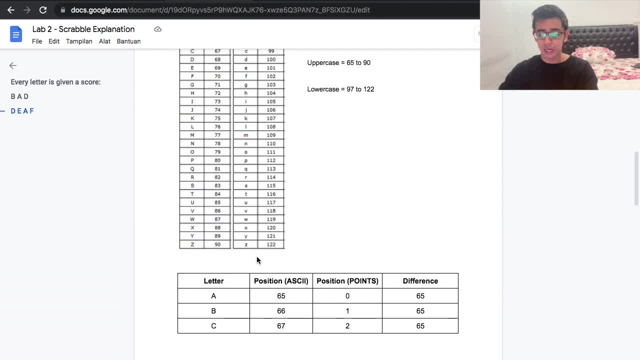 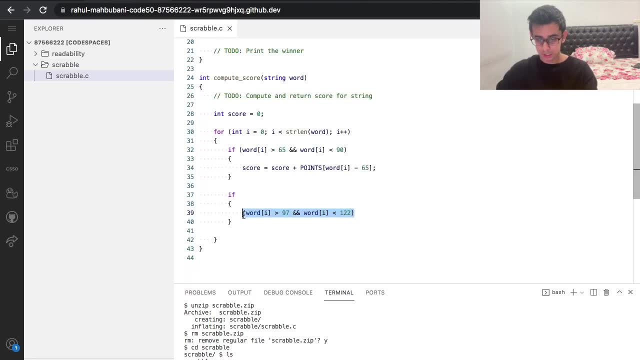 is. let's check real quick: whatever lowercase z is, lowercase z is 1 2 2. okay, so 1 2 2. then so if it's greater than 97 and less than 1 to 2, which is basically saying if it's an, 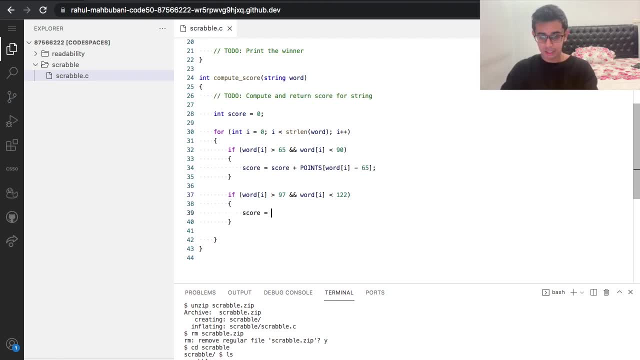 uppercase letter, then we need to do score equals score, this way to update the score plus points, and the index it should take in the points array is whatever the index is in ascii minus 97, right, because lowercase a is 97. but here it's just it feels a little bit complicated. here we're saying like greater. 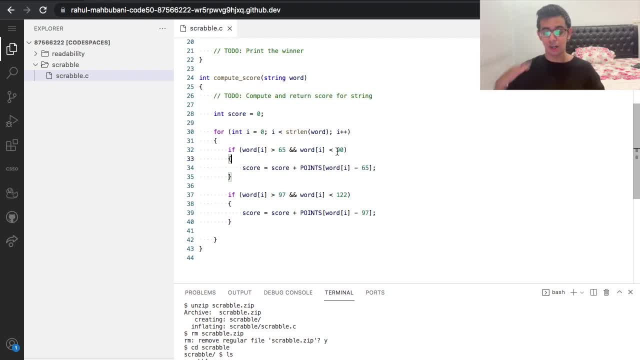 than 65, less than 90, and this is completely correct. so far, logically, it's correct. but what if there was a simpler way to say if it was uppercase and if it was lowercase, rather than checking the ascii values and doing all that? well, turns out there is a way to do that. 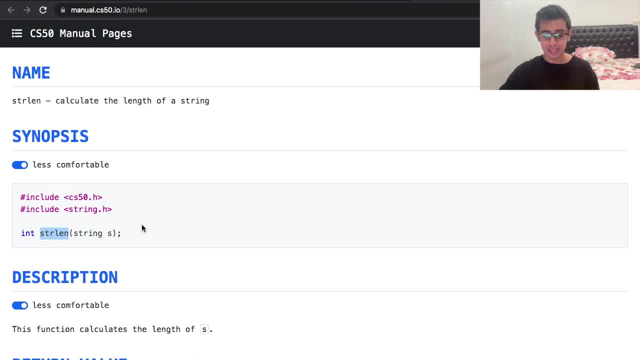 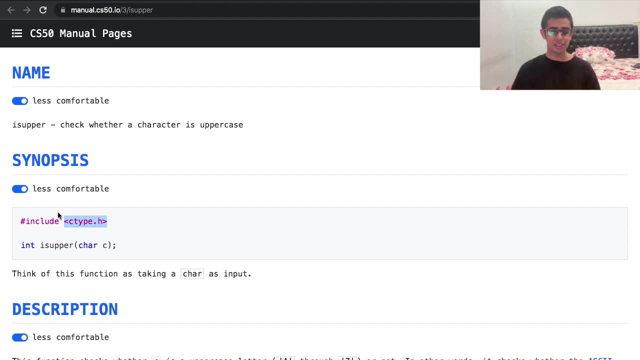 and the way we do that is using this function right here. so it's called is upper and it's under the header ctypeh, and you wouldn't know this unless you actually went through the entire cs50 manual, so don't worry at all. so, but it turns out there is a function called is upper which checks whether 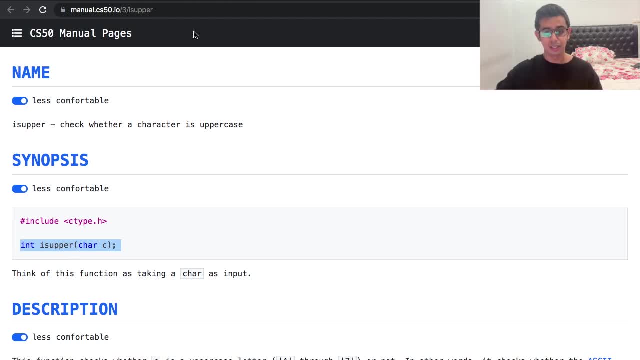 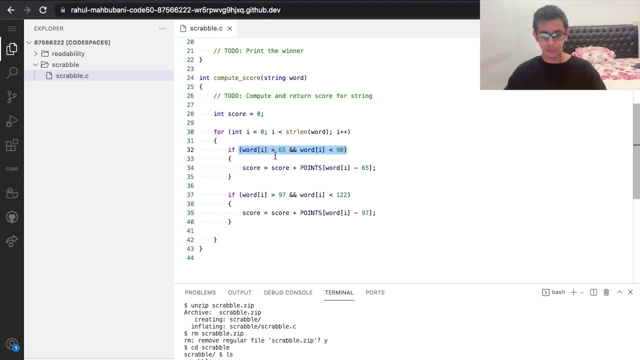 or not the function is uh, whether or not the letter is uppercase. so rather than doing this whole long thing, rather than saying between 65 and 90, greater than 65, less than 9, doing all this, what we can simply do is try to do the same thing here. so let's say we want to do the same thing here. 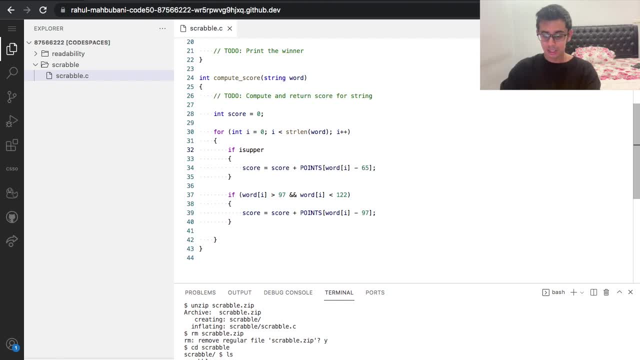 is. replace it with: the function is upper, if is upper word. so it checks whether the index is uppercase or not, whether the character in that index uppercase or not, and if is, it'll execute this. so it's the exact same thing functionally, but just it's simpler right. if we can use the function, why do we have to reinvent? 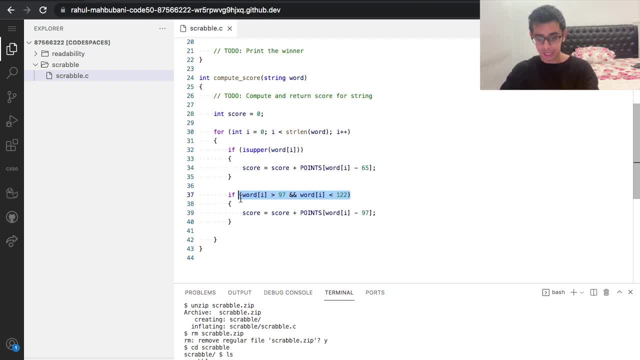 the wheel and do it all over again, so we can do the same thing here. if is lower for this one. that's the name of the function word. i right, if you do it the previous way, it's correct as well. if you did this way, it's correct as well. this is just simpler right. 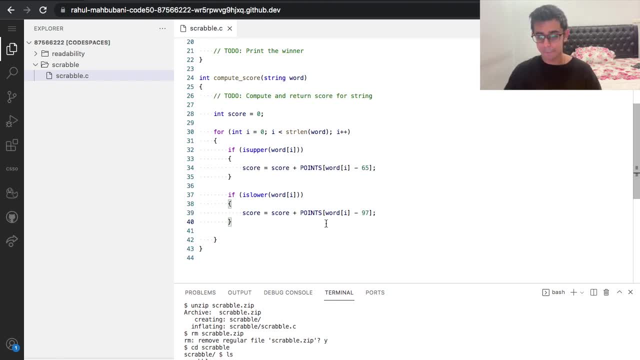 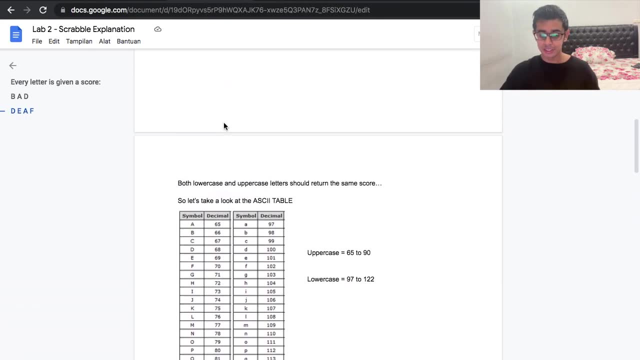 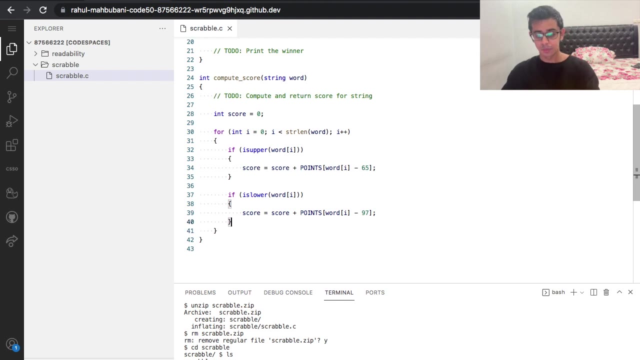 so we've done all this so far, but, uh, actually we don't just want to return the score, we don't just want to print the score, we need to. we need to calculate the score and then we need to print out the winner, right? so what we need to do here is return score, right? um, okay, 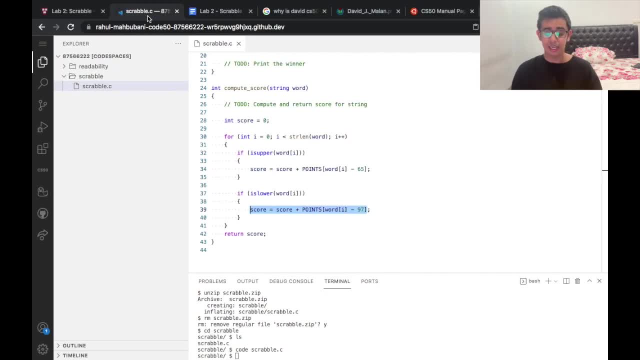 i hope everything's clear so far. if you don't understand anything, please rewind, or if anything's unclear up to this point, please leave a comment down below and i'll be sure to answer every single comment. right, but hopefully everything's clear and here we've calculated the. 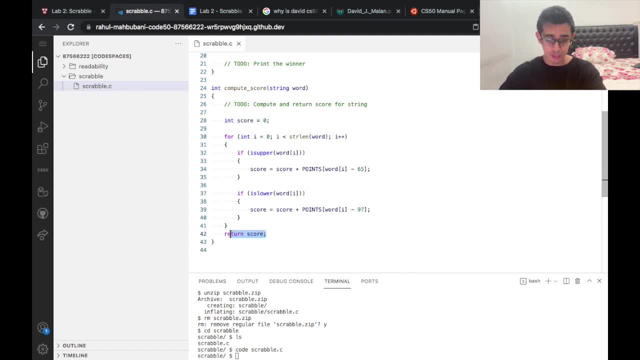 number of points, but we don't want to print the score here. we want to return the score and we want to print the winner instead. so here it's very simple, right? so what we do is simply print f. sorry, we need conditions, right? so if score one is greater than score two, 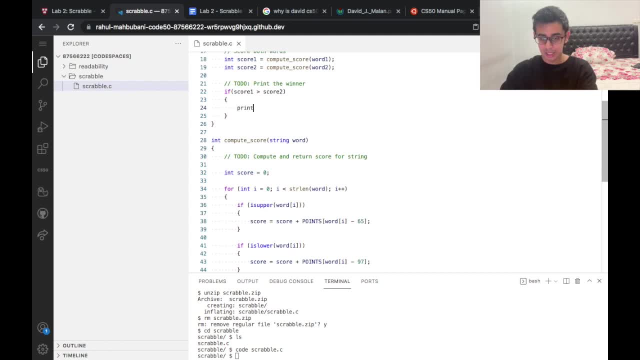 we need to print? what do we need to print? player one wins- right. player one wins, and these are according to the instructions. so we need to print f. sorry, we need conditions right. so if score one is greater than score two, we need to print: player one wins and these are according to the instructions. 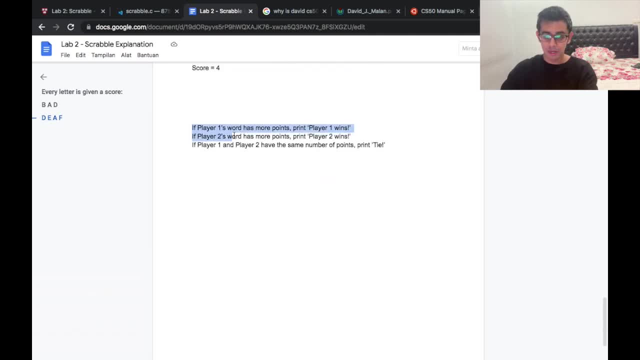 on cs50 themselves. right? so if player, if player one's word has more points, print player one wins. if player two has more points, print player two wins. and if player one and player two have the same number of points, print tie. okay, this is what they tell us to do, so this is the 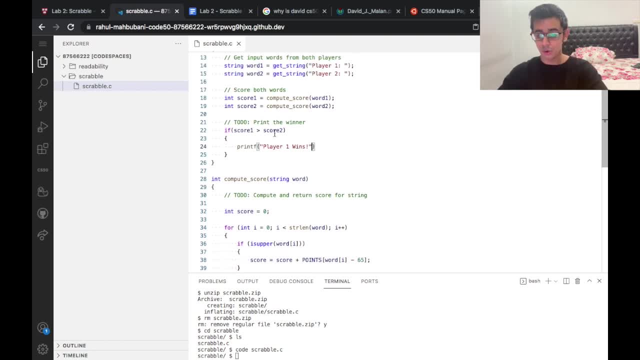 way to do it right in code. right, if score one is greater than score two, print player one wins. this makes a lot, just makes logical sense. else, if score two is greater than score two, greater than score one, what do we do? what do we need to print here? print player two wins. 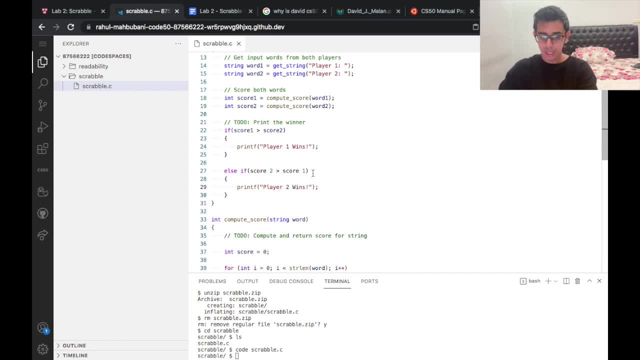 player, two wins, okay. and there's a third scenario here. right, if it's a tie, so else print tie, right. and here we can write the condition: if score two is equal to score one, uh, but we don't have to write it, because if it's not this, if it's if one is not greater than two. 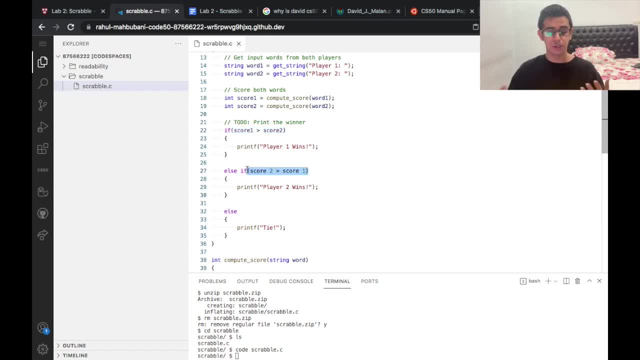 and two is not greater than one. it's understood that one is equal to two, so we have the same player one and player two at the same number of points. so we can write it. we can write here else if um score one is equal to score two, but we don't have to because it's understood logically. 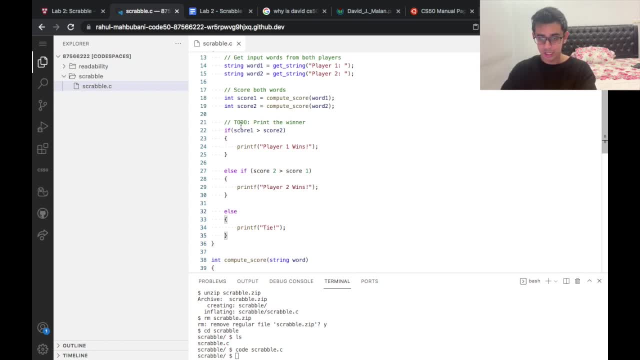 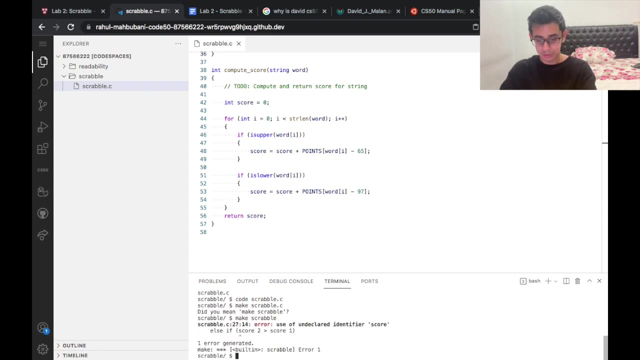 right. so everything here makes sense so far, and let's just go ahead and compile the program. see if we did anything wrong. make scrabble, dot c- oh sorry, make scrabble, not mixture this. i compile, make scrabble- oh, one error generator here. oh okay, so in line 27 there is an error and here the problem is okay. so we can see here that the 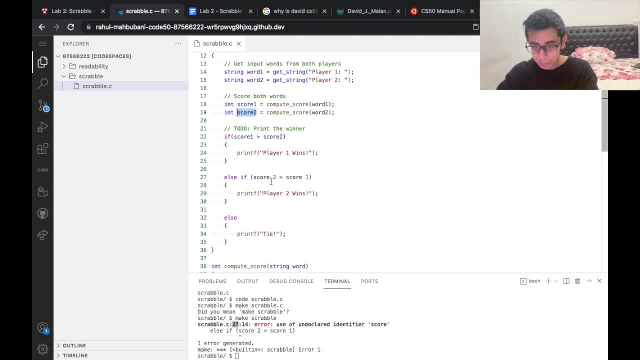 variable is defined as score two, whereas here i accidentally put a space, so that's not going to count that as it um as the variable. so it needs to be exactly what you do, what the variable is, you need to write it exactly. we can't accidentally put a space here. space there completely changes the meaning. 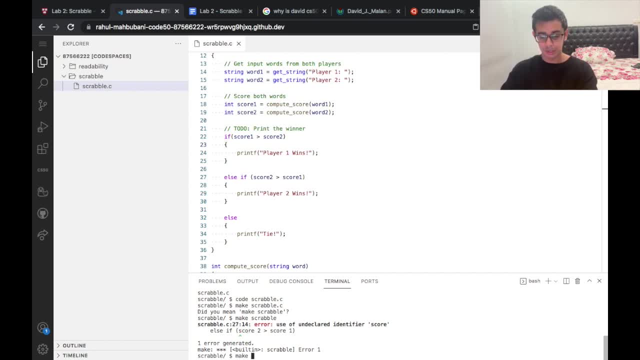 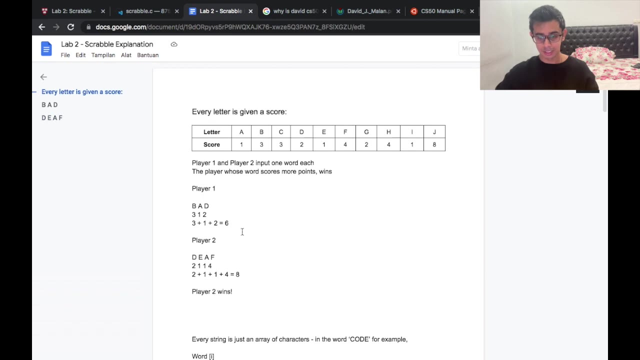 and, as you can see, it gave us an error there, so that was just a silly mistake on my part. so let's try to compile again, make scrabble okay. let's try dot slash scrabble to run it okay. it asked me player one. and let's just go back to our earlier example here: bad, right. player one says bad. 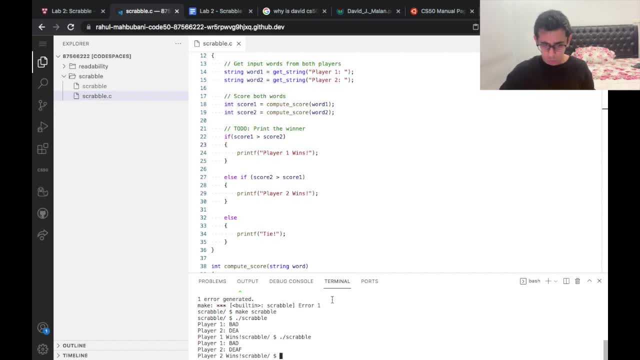 says: dev player two wins, okay, oh, one small thing here is that um, the prompt starts in the same line, so let's just make a new line here. we do that by doing backslash n, so every time we print something we want it to always move to the new line. after that, it's just. 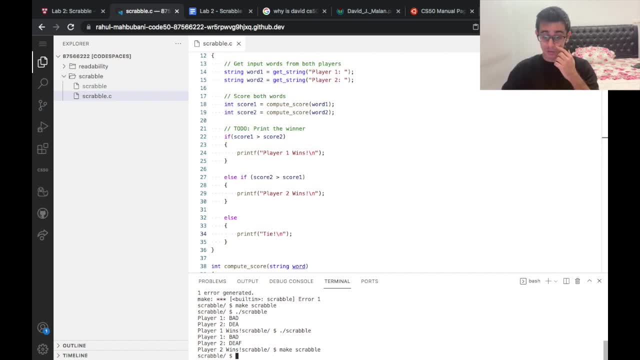 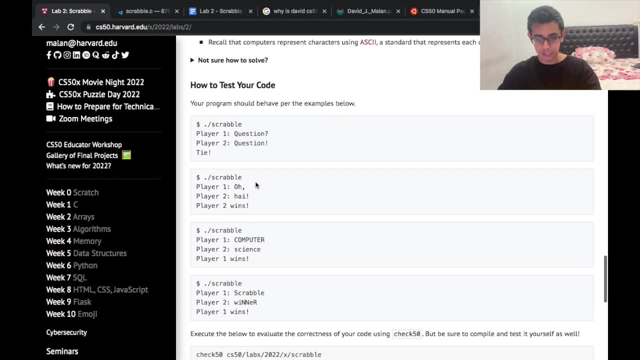 it's still correct. the code itself is correct. it's just that, uh, for neatness sake, you know, for style's sake. so let's see what they tell us to check here, what cs50 themselves want us to check. so let's check the word computer player. one says the word computer. 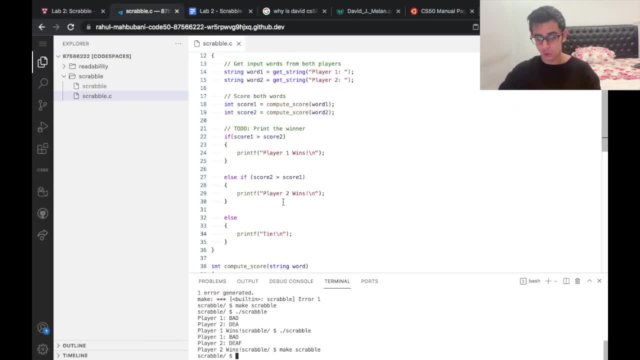 in all caps. and remember we've already accounted for the uppercase and lowercase over here. if is upper then minus 65 is, if lower then minus 97. so we've already accounted for that. so it shouldn't be a problem here that they tell us to check computer with all caps. 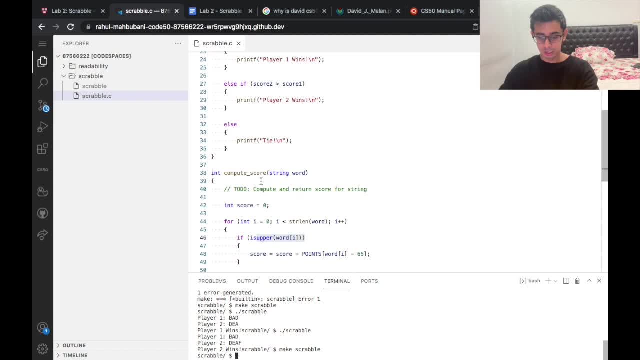 and science with all lowercase. so let's make scrabble, let's run it dot scrabble. player one puts in the word computer and player two puts in the word science and player one wins. and, as it should print, player one wins. okay, everything's correct so far. 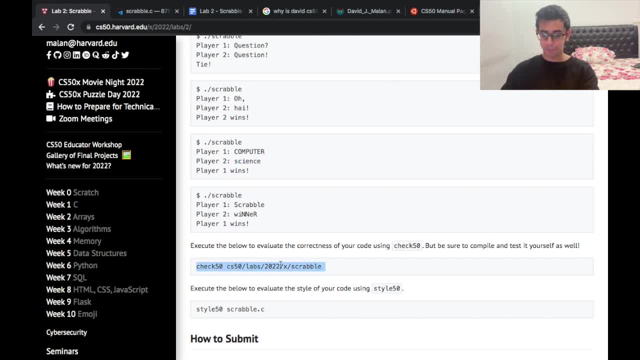 let's just go ahead and check, just copying and pasting this code here to check whether or not it's correct. and this is um from the from the original file itself, right? this is the link i'll put in the description. it's a. it's cs50's official. 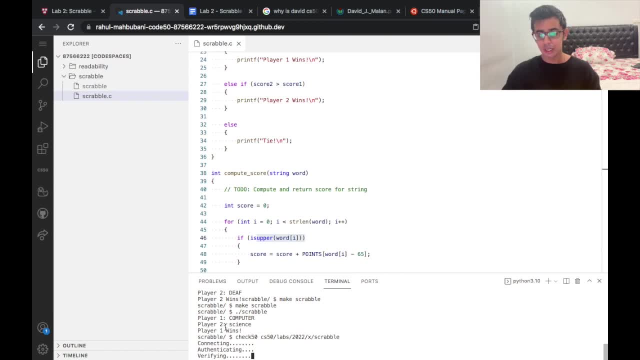 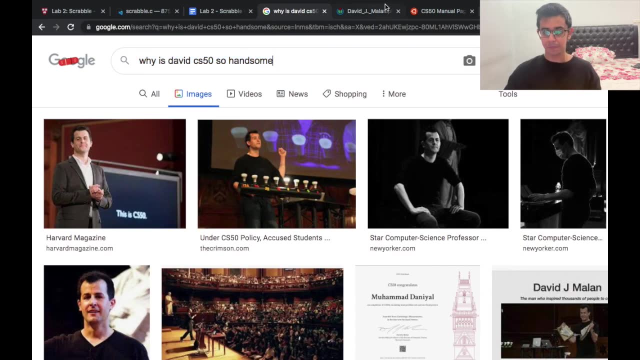 link to explain what scrabble is. i'm just going to go ahead and check here, and while we're doing that, guys always remember to check the manual. oh, wrong tabs, oops. um, right, so we use some functions here. they're a part of the manual, right, but they? 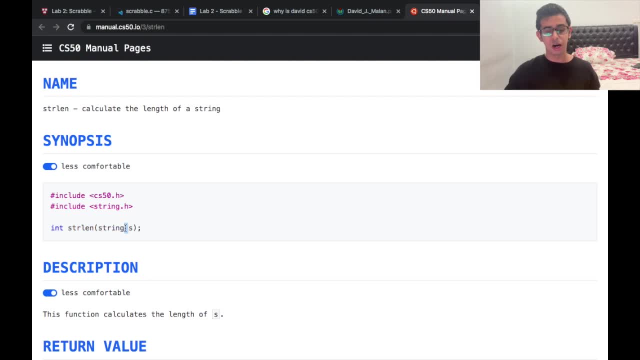 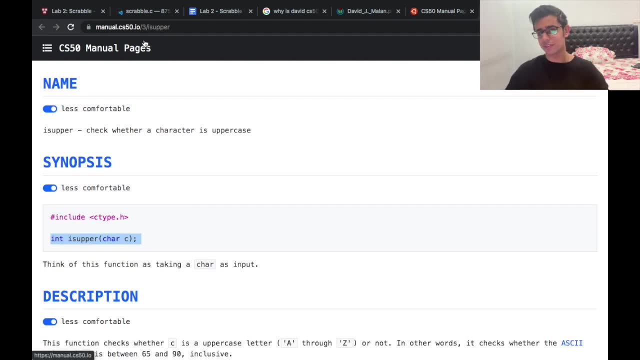 didn't explicitly explain it in the lecture. so, um, in your free time, just go over the function right, it can save us a lot of time, like we did the is upper. we had to do a whole bunch of things from ascii and less than 97, greater than 1-2-2, all that stuff. 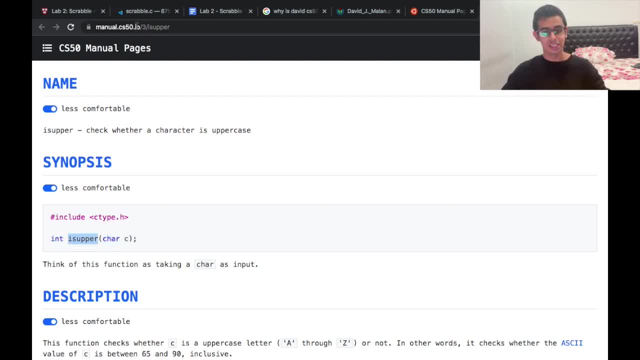 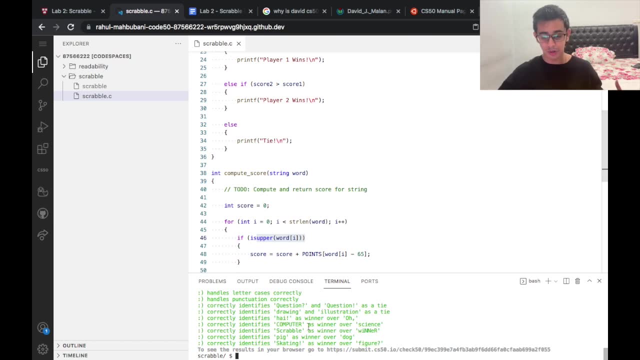 it could have been saved if we simply knew about the function called isUpper right. So it's worth it to go through the whole thing, go through everything and kind of get a feel for all the functions and everything, so that we can save time in the future. 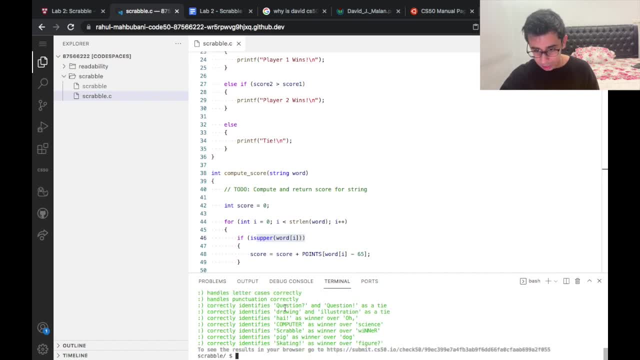 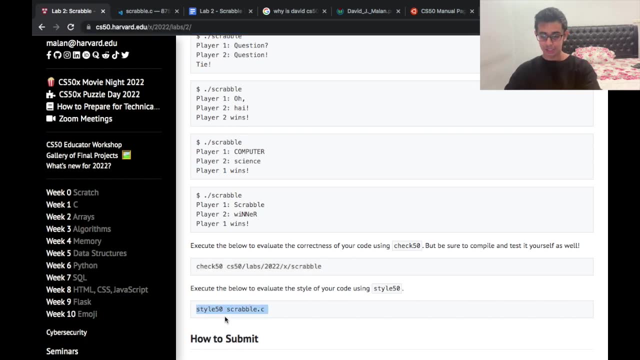 And we can see here: it's done checking and everything's green, which means everything's good, Everything's correct. And if you want to maximize your points, you can also put in this code to check the style of your code, right.